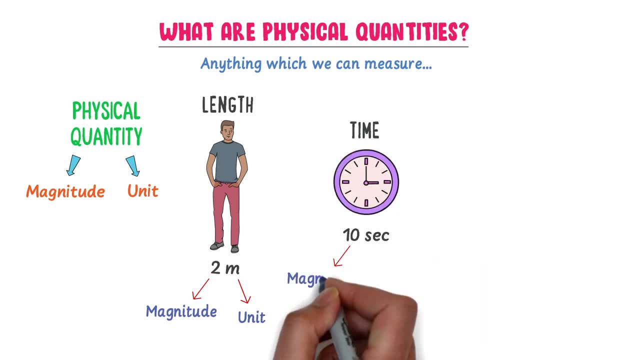 time is 10 second. Here 10 is the size or magnitude, while second is the unit of time. We can measure the time, So it is a physical quantity. Thirdly, consider vegetable or fruits. Let the mass of vegetable is 3 kg. Here 3 is the size or 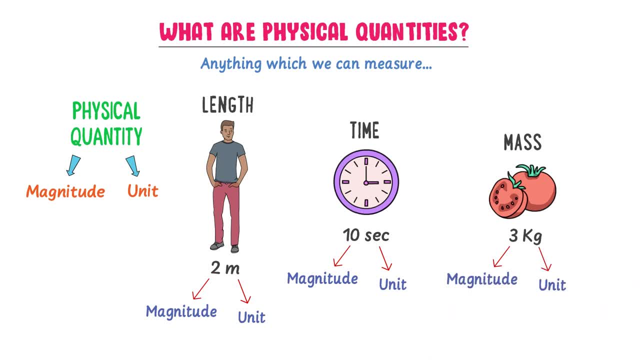 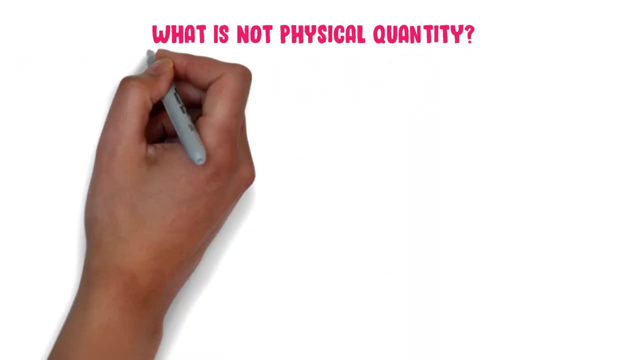 magnitude. kg is the unit of mass. We can measure mass of anything, So it is a physical quantity. So remember that anything which we can measure is called physical quantity. Now let me teach you one bonus question. What is not a physical quantity? Well, any number having no unit. 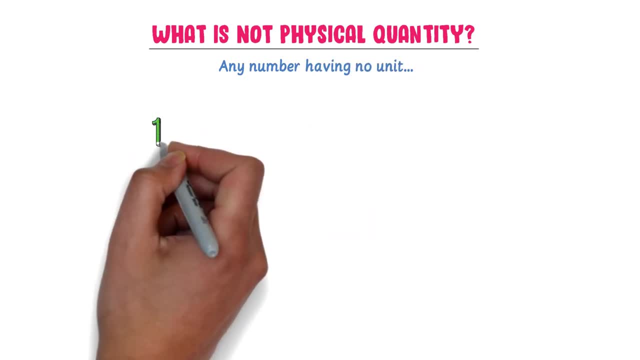 is not a physical quantity. For example, consider 12, 13, 14.. 12 is only number, 13 is also only number and 14 is also only number having no unit. So we say that these are not physical quantities. 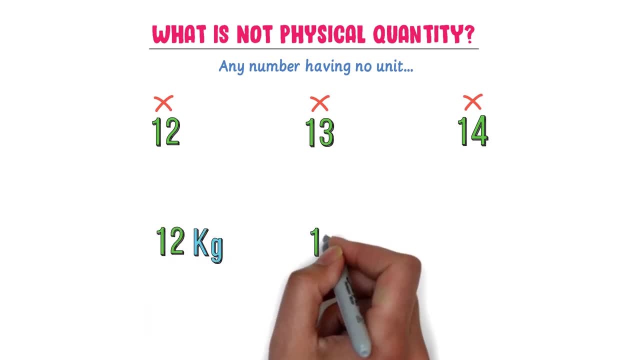 On the other hand, if I write 12 kg, 13, second, 14 meter, Here kg is the unit of mass, second is the unit of the time and meter is the unit of length. So 12 kg is a physical quantity. 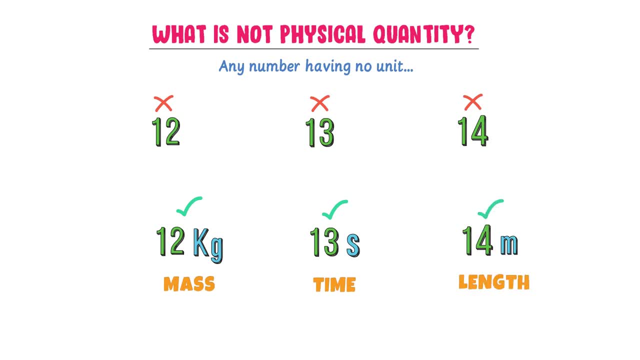 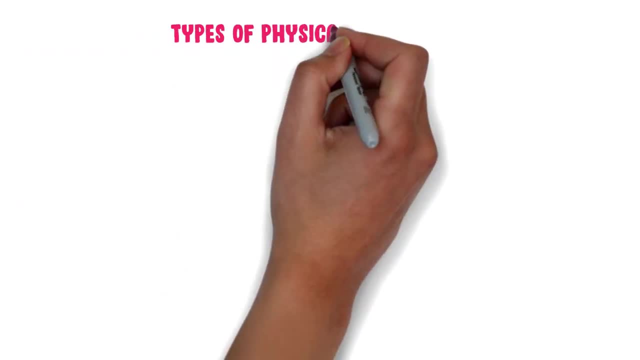 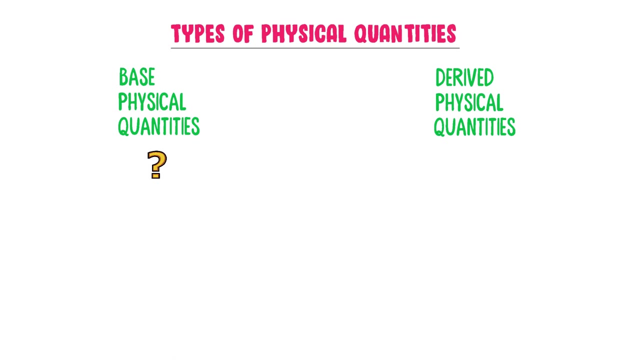 13, second is a physical quantity and 14 meter is the physical quantity. Let's noted down this bonus question. Remember that physical quantities are divided into best physical quantities and derived physical quantities. Now, but what are best physical quantities? Well, the seven physical quantities. in terms of which other physical 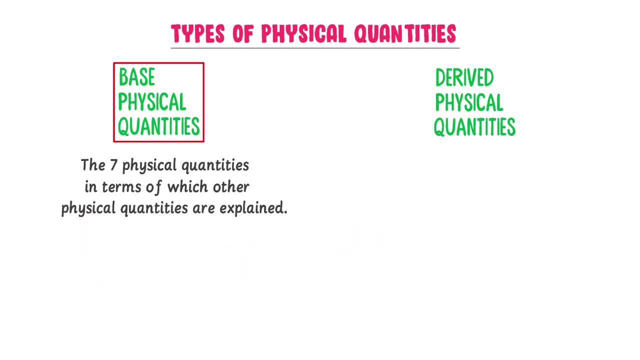 quantities are explained are called base physical quantities. For example, length, time, mass, etc. are all base physical quantities. Now, what are derived physical quantities? Well, those physical quantities that are derived from base physical quantities are called derived physical quantities. For example, I divide length by time. When we divide these two base physical quantities, 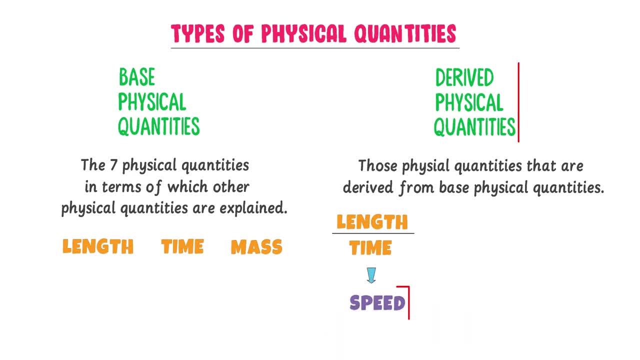 we get another physical quantity like speed, which is derived physical quantity. Secondly, let consider length into length, which is equal to area. Here, when we multiply two base physical quantities, we get derived quantity like area. Thirdly, consider mass into speed is equal to area. Here, when we multiply two base physical quantities, we get derived quantity. 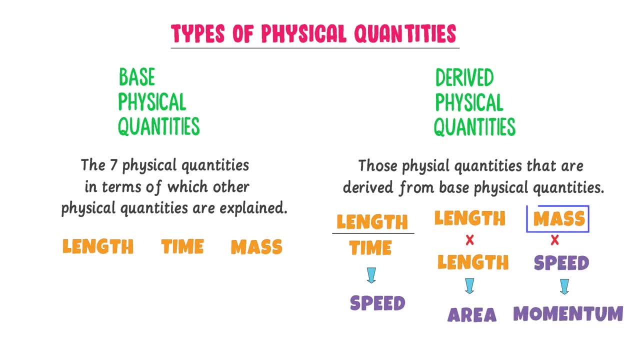 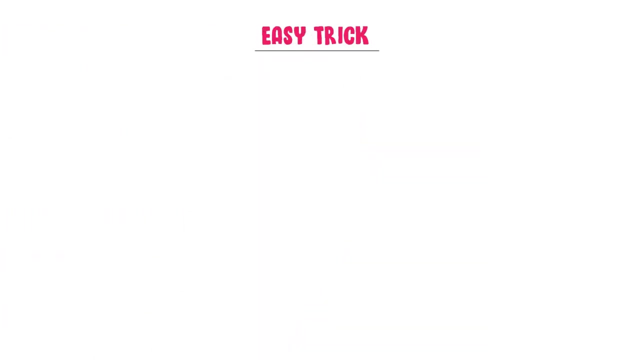 equal to momentum. Here mass is base physical quantity, while speed is derived physical quantity. Sometime when we multiply base and derived physical quantity, again we get derived quantity like momentum. Just remember about base physical quantities and derived physical quantities. Now let me teach you my personal trick to remember base physical quantities and derived physical. 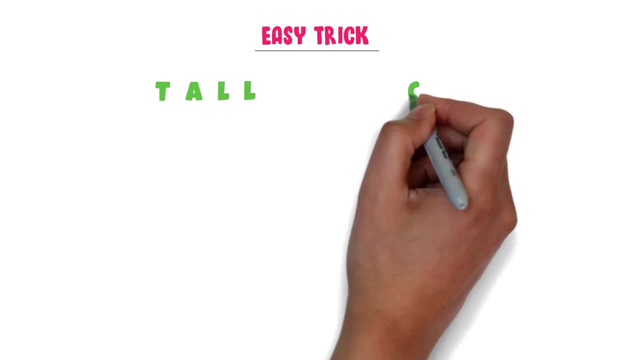 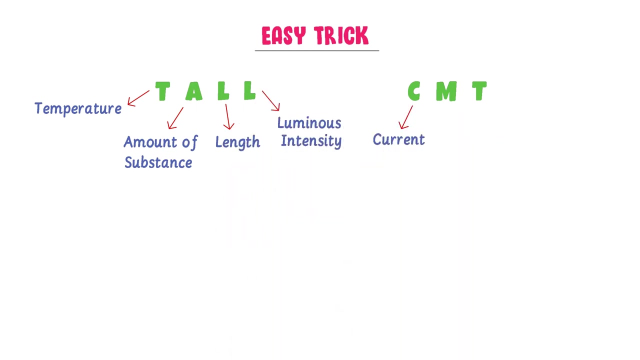 quantities. I always write tall cmt. This t stands for temperature. this a stands for amount of substance. l stands for length. this l stands for light intensity. c stands for current. m stands for mass, t stands for time. These are the seven base physical quantities. Except these seven base, 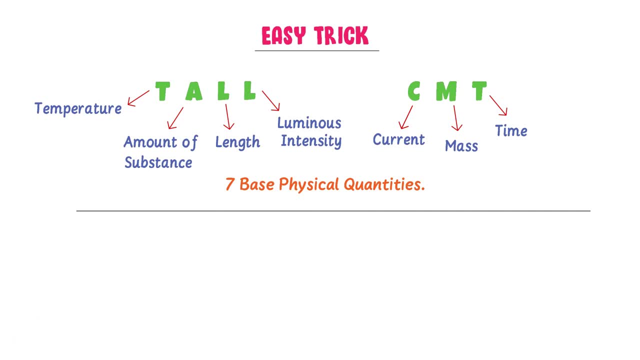 quantities. all physical quantities are the same, So I always write tall cmt. This t stands for different types of time. sac for young T. take them Now. how about the number of physical quantities? Let me write this derived quantity: light intensity is present in this list, so it is base physical quantity. 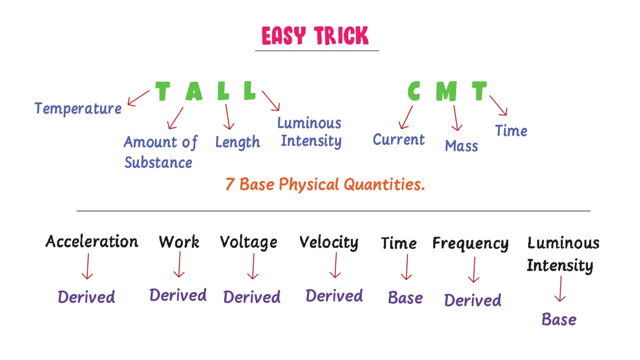 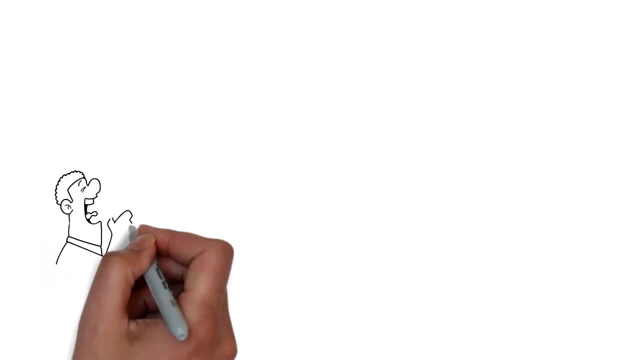 Thus, by this way, we can easily spot the base physical quantity and the derived physical quantity in any question. Finally, let me introduce the new concept of physics world in my upcoming lectures. In our daily life we can see different sign boards like speed limit. 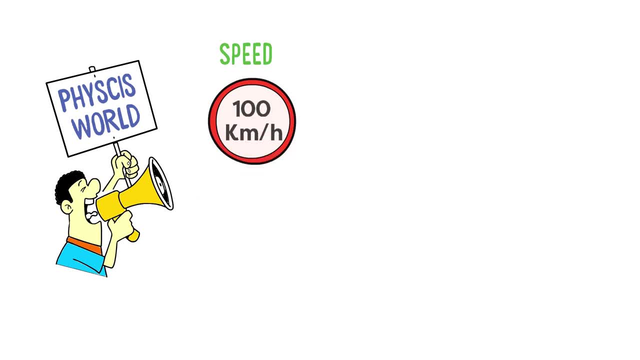 in which it is written as 100 km per hour. In this case, 100 is the magnitude or size. km per hour is the unit of speed. So this is a physical quantity because it has magnitude and unit. Let me ask you: is it a base or derived quantity? Well, it is a derived physical quantity.